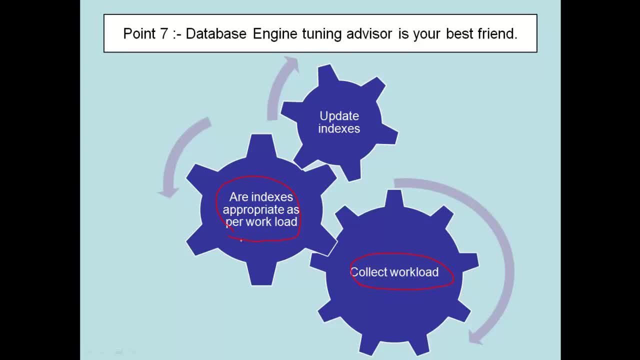 around something else to find that where the SQL performance can be improved. If they are not, then you would like to go and update the indexes as per the workload. It's a three-step process. First you collect the workload. Second, you analyze if the indexes are. 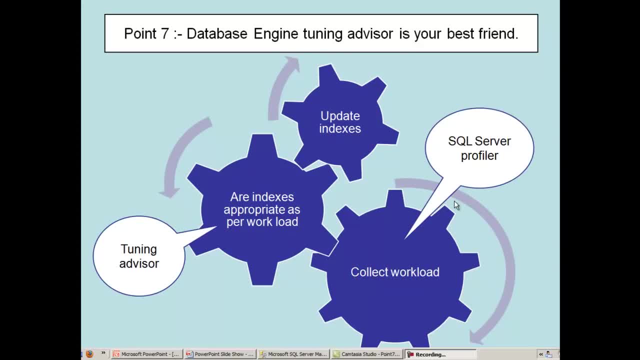 appropriate as per the workload and then you update your indexes. Both of these activities, ie collection of the workload as well as to analyze if the indexes are appropriate as per the workload, cannot be a manual process. You would like to use some kind of tool for this because, in case you are working on a database with 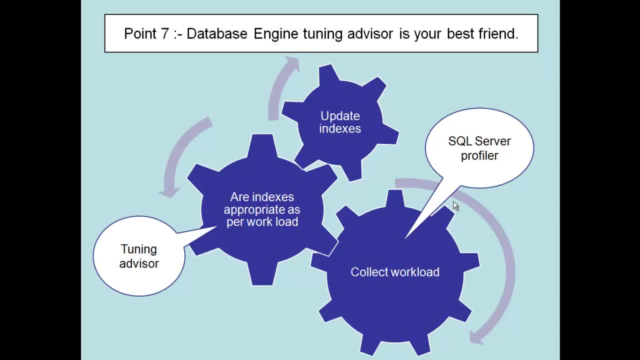 has thousands of tables and lot of stored procedures and it has lot of transactions. it's humanly not possible to go and analyze that workload and come up with accurate index plan. For the same, what SQL Server has done is it has provided two tools. one is the SQL Profiler. 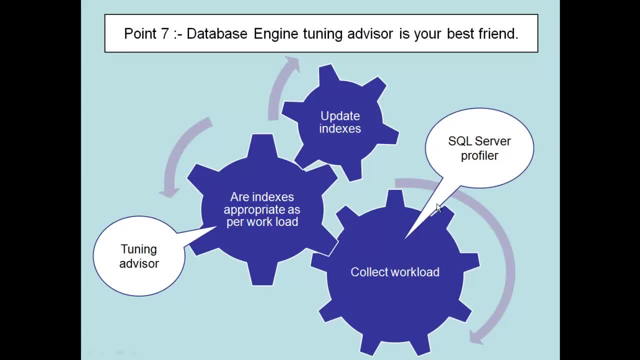 and the other one is the Tuning Advisor. The SQL Profiler will help us to automate the collection of the workload, while the Tuning Advisor will help us to take the workload which has been gathered by the SQL Profiler and come up with appropriate indexes. 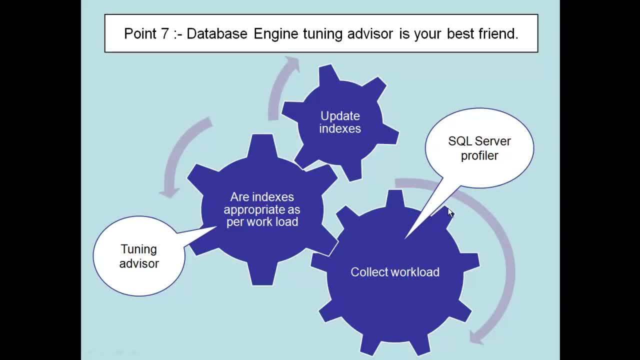 Let's do a small practical demonstration here, and in this demonstration what we will do is we will pick up a database, we will pick up couple of tables from the database and we will first collect the workload by using SQL Server Profiler and then we will run the 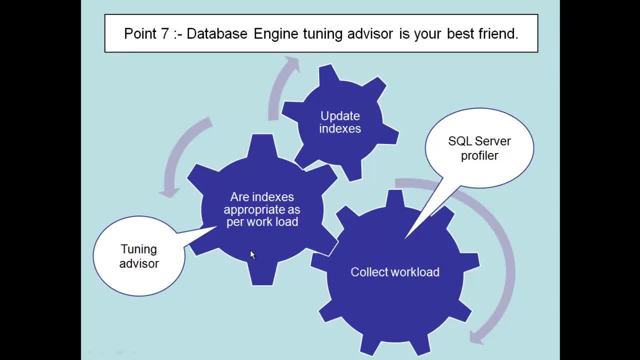 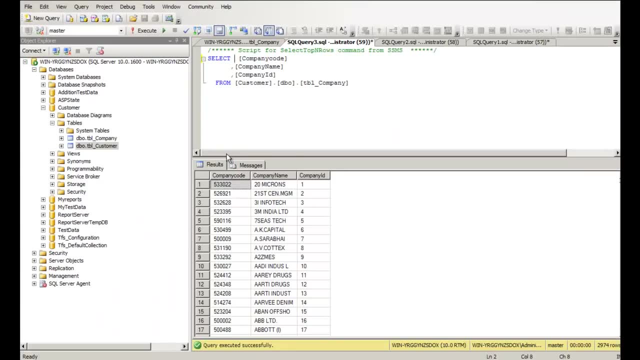 Tuning Advisor on the workload to see that if the indexes are appropriate or not, and then we will see that how the performance basically improves after using the Tuning Advisor, In order to demonstrate how to use the Profiler as well as the Tuning Advisor. 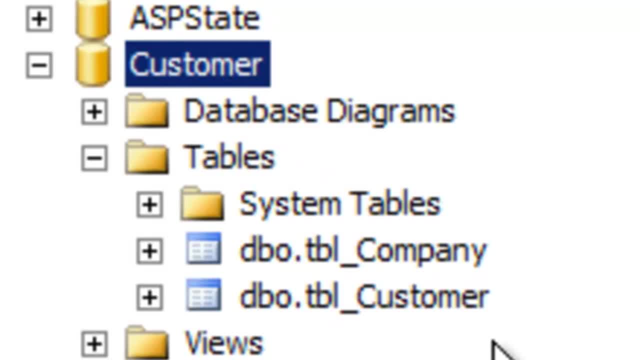 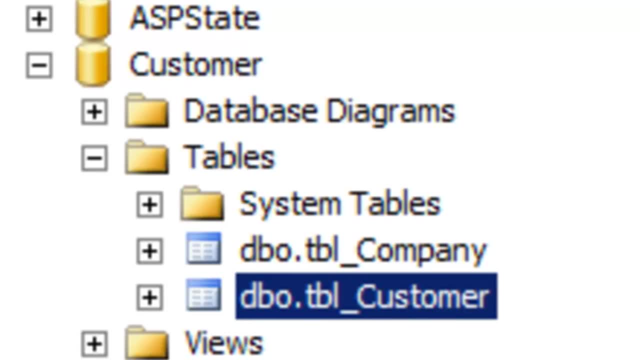 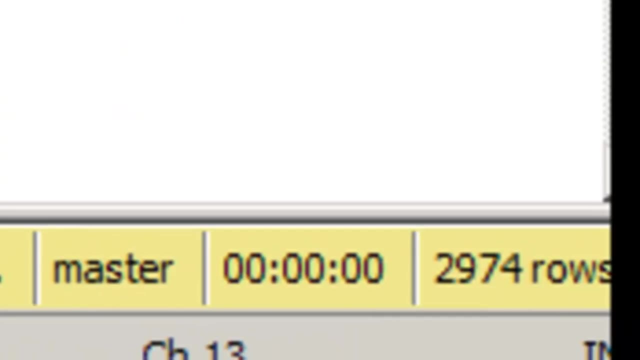 here's a simple sample we are going to do. A customer database has two tables here. one is the tbl underscore company and the other one is the tbl underscore customer. The tbl underscore company has approximately 3000 records, so 2974 records it has, while the tbl underscore customer it has like hardly 5 or 6. 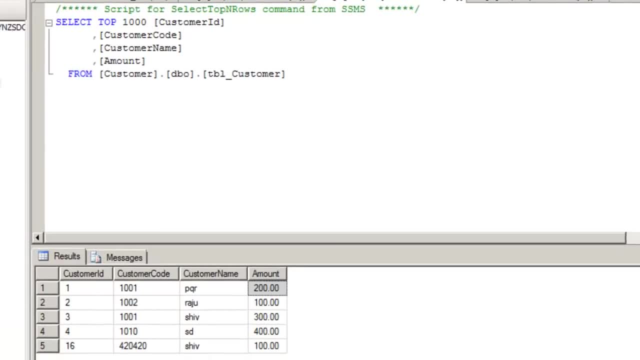 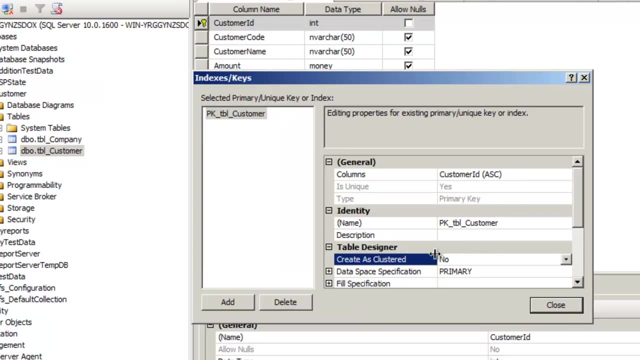 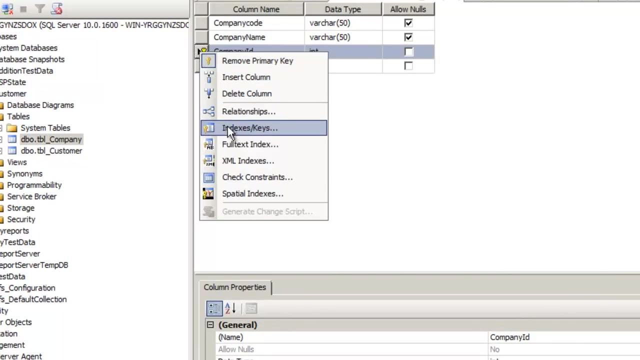 records, Both of these tables don't have indexes. so, for example, if I go to tbl underscore customer and if I see for the indexes, currently there is no index for now, and the same for tbl underscore company- currently there is no index for now. If I go to the design and if I go to the indexes, currently there is no indexes on both of. 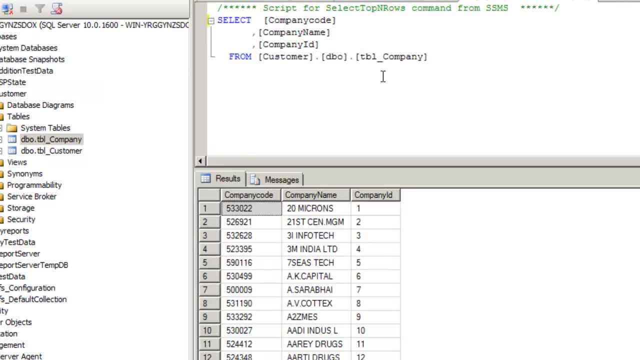 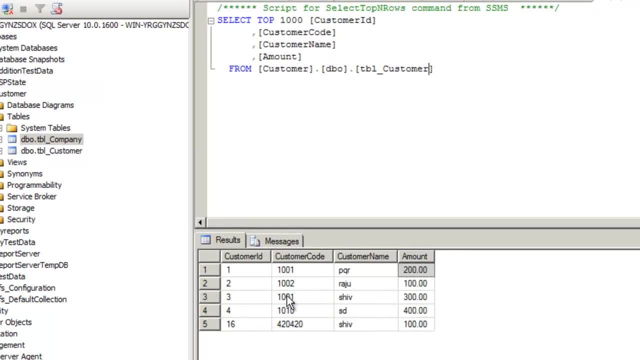 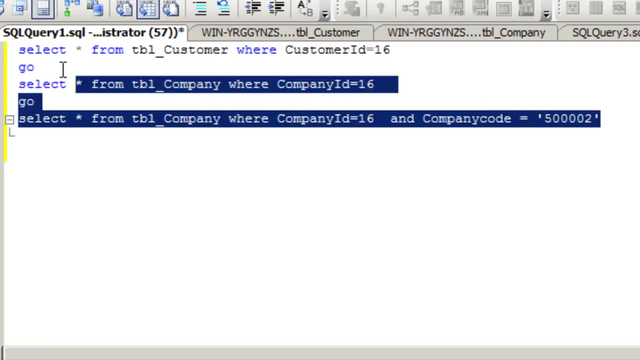 these tables. One of the tables, that is, the tbl underscore company, has approximately 3000 records, 2974, and the tbl underscore customer has five records. On these two tables, following kind of SQL queries are fired from the, From an ASPNET application or from a C-sharp application: 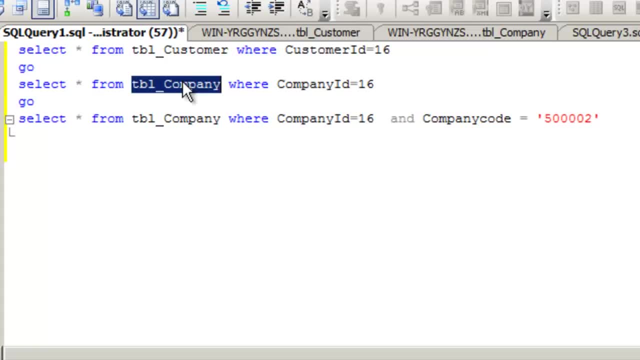 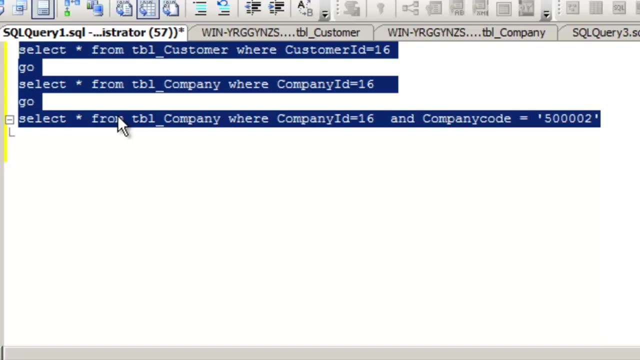 sometimes the TBL customer is searched by CustomerId, the TBL company is searched by CompanyId and sometimes the TBL company is also searched by CompanyId as well as the CompanyCode. These are the frequently fired select statements on these two tables. I will iterate one point. 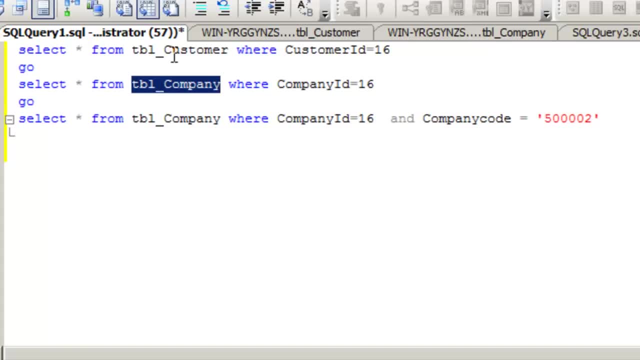 TBL company is having approximately 3000 records, while the TBL customer just has 5 records. We will use this select nature and we will generate a workload file using the SQL Server Profiler. We will fire the select statement at the backend. run the profiler. 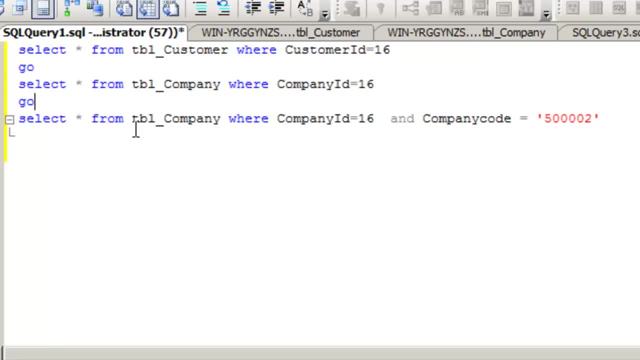 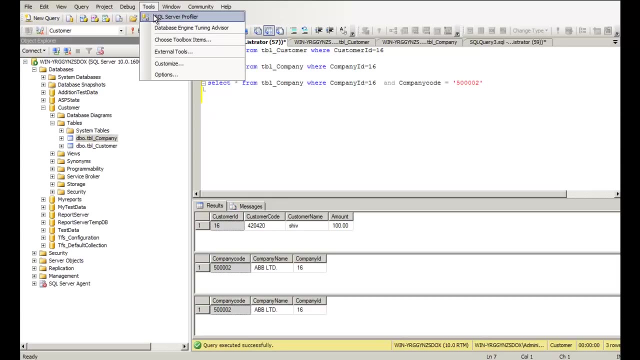 and will first generate a workload file. Once we generate the workload file, we will take that workload file and we will use the tuning advisor to see what kind of indexes it suggests us. Let's first run the profiler here. Click on Tools, Click on SQL Server Profiler. 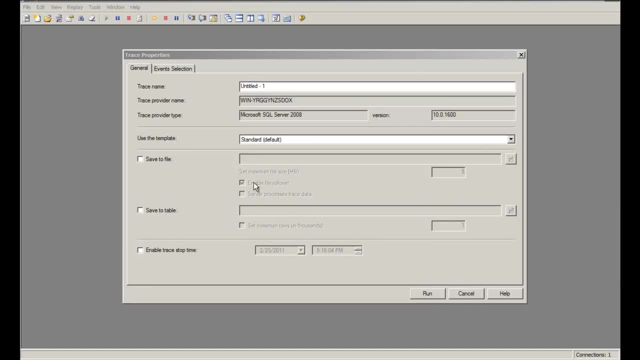 and click on Connect. Before we run this tool, let me talk about what exactly is a SQL Server Profiler. SQL Server Profiler is a nice tool which helps to capture what kind of SQL statements are fired on your SQL Server. When we click on Run, we can see that it has started capturing a lot of. 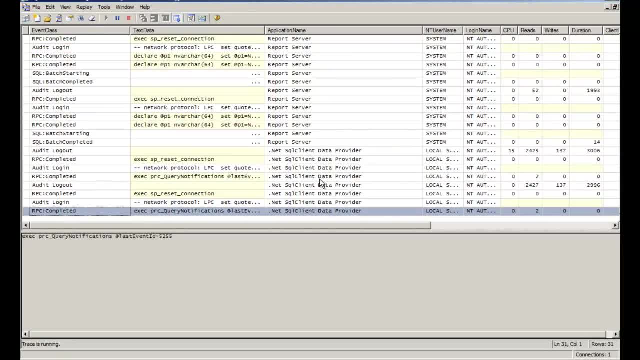 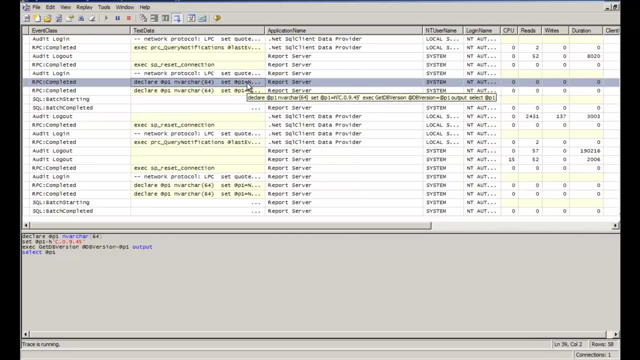 a lot of events here or it has started capturing a lot of activities which are happening on the database. For example, we can see that it's capturing that there are some SQL statements which are getting fired on report server, There are some SQL statements which are probably notification SQL statements, etc. 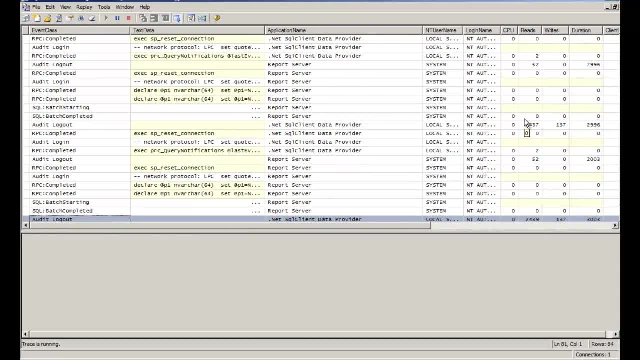 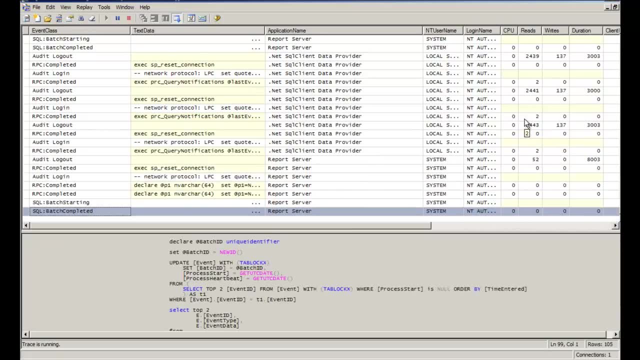 In other words, SQL Server Profiler is nothing, but it's like a listener tool which sits at the backend and quietly hears what kind of SQL statements are getting fired on your database. This tool is heavily used when we want to debug an application, when we want to know 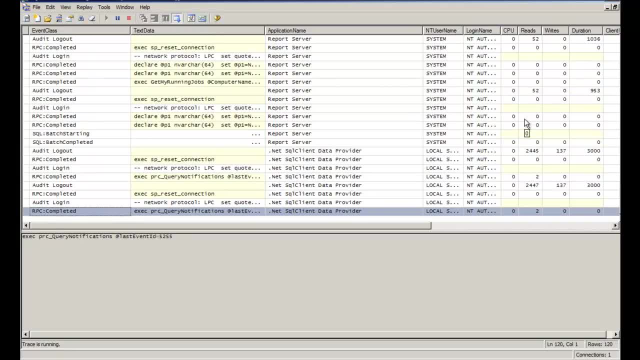 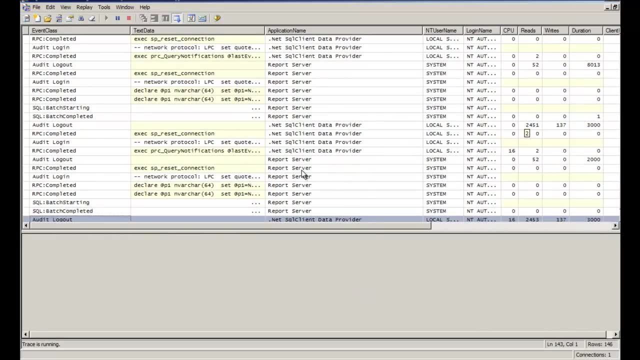 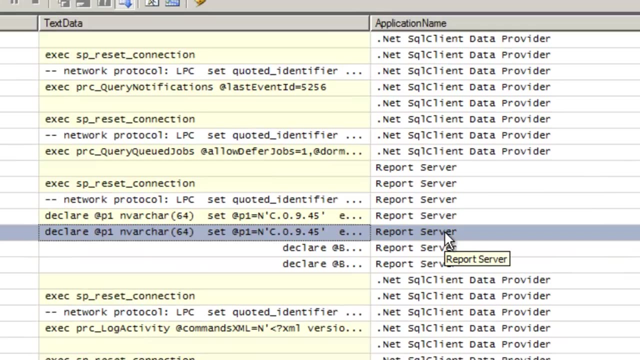 what kind of select queries are fired and what kind of data is been sent to the select queries or to your SQL queries. Now that we are running this tool, there is one big problem here. The problem is that it is capturing lot of SQL statements which are probably not relevant to us. 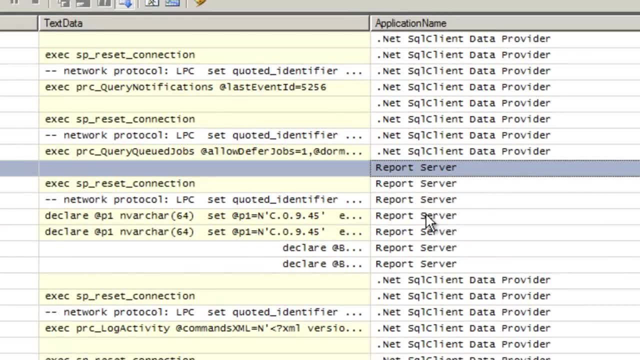 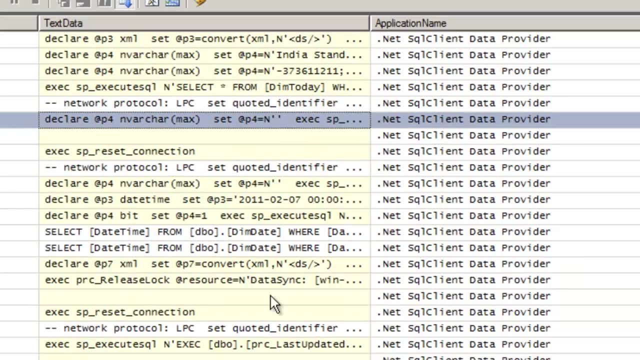 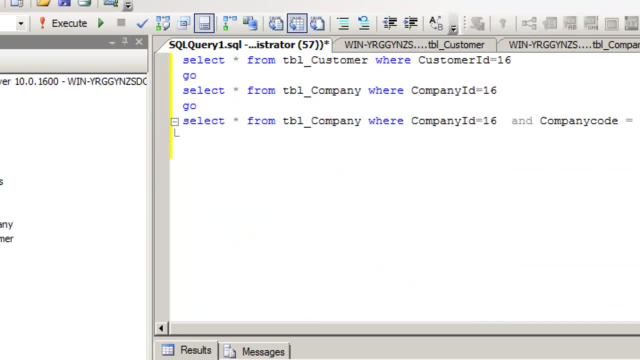 For example, we can see that it is capturing SQL statements which are fired on report server. it is capturing some SQL statements which are fired on, like for the notifications services, for the log purpose, etc. Our main goal is we want to basically go and see that how we can improve performance on the customer database. 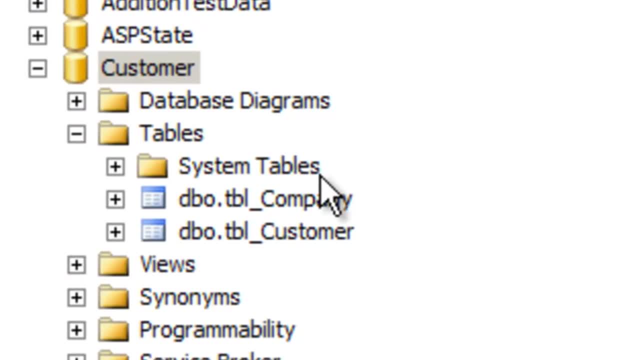 We are not really interested in hearing what's happening on the report server or we do not want to capture the workload which is not relevant to our tuning currently. What I am interested currently is I just want to hear SQL statement which are getting fired on customer database and I just want to take those SQL statements. 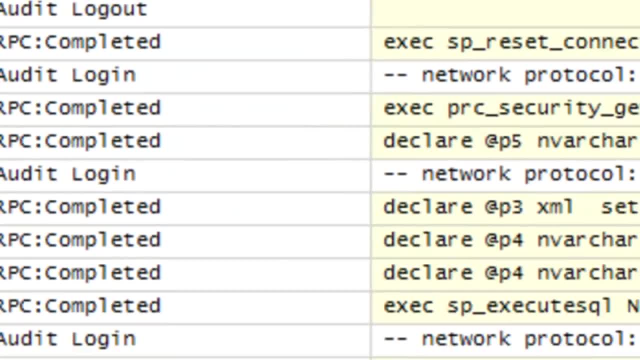 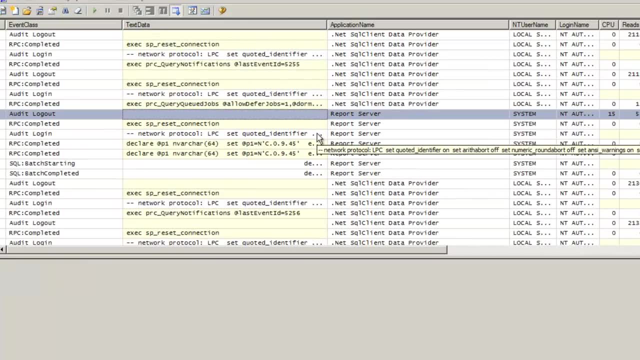 as my workload and then do the fine tuning. In other words, I would like to remove this noise over here which is not relevant or probably it would not add any value for my tuning activity. In order to remove this noise, what we can do is we can put up a filter here. 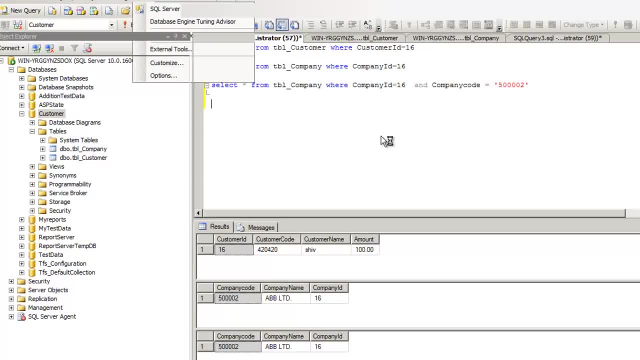 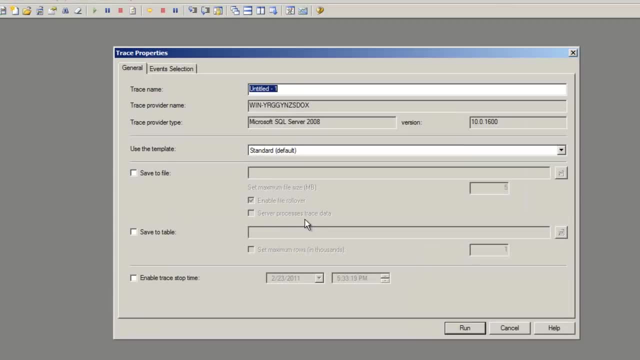 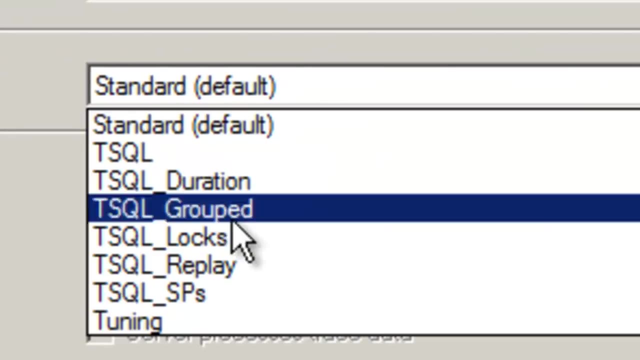 Go back again and fire the SQL profiler and this time put up a filter. There goes my SQL sub profiler Connect. Now, because our activity is more relevant towards tuning, what we will do is that we will not select the standard default template, but we will select the tuning template. 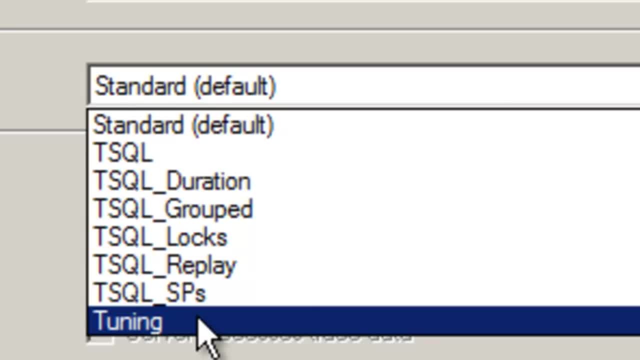 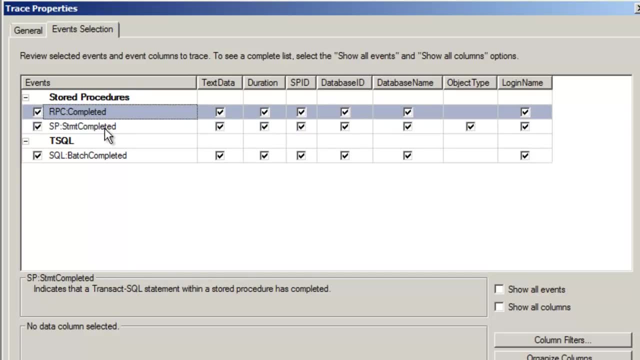 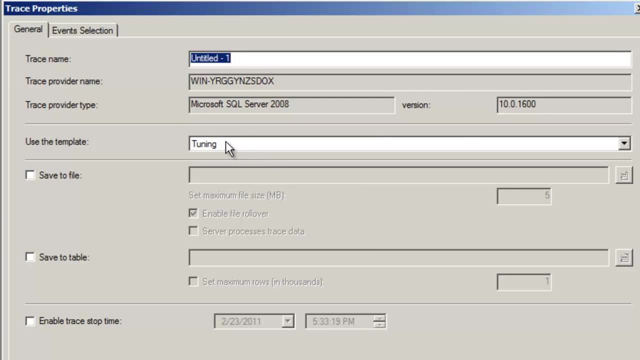 This tuning template is provided by SQL server itself and basically, if you click on the tuning template, you will see that basically it just listens to the SQL statements and the RPC statements. That's what we want. First, go and select the tuning template and second, we would like to go and 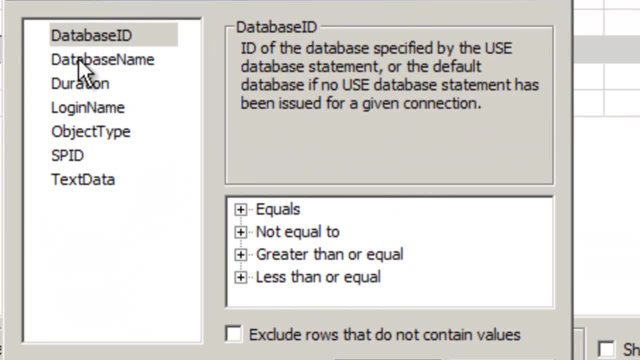 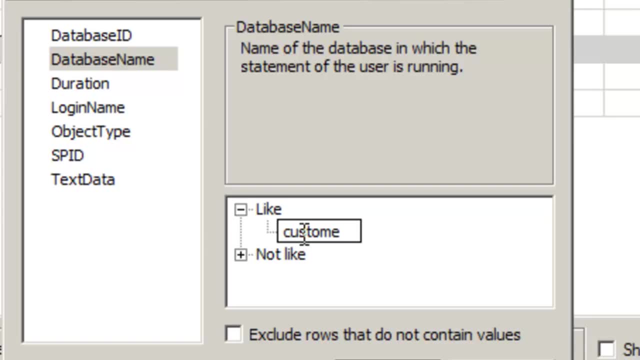 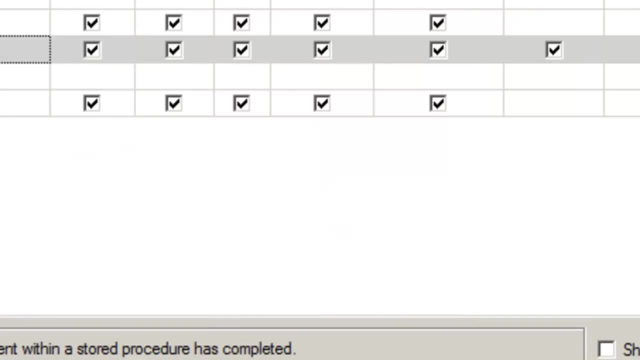 put a filter- Go to Columns filter here- and let me say that I am just interested to here SQL statements which are fired on customer tables. Customer database. My database name is customer. What will happen is that it will not. it will no more hear to other databases like report server or any other database. 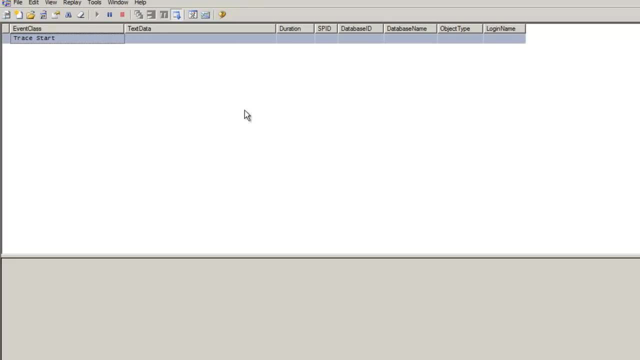 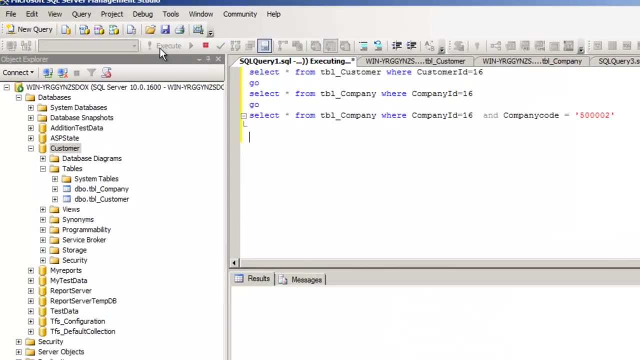 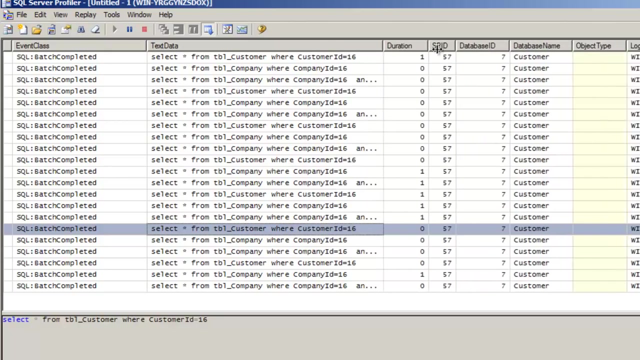 but it will only capture SQL statements which are relevant to the customer database. Now we will go and fire the SQL statements which we had written. so I am firing it couple of times here and you can see that my SQL server profiler has captured the load over here. 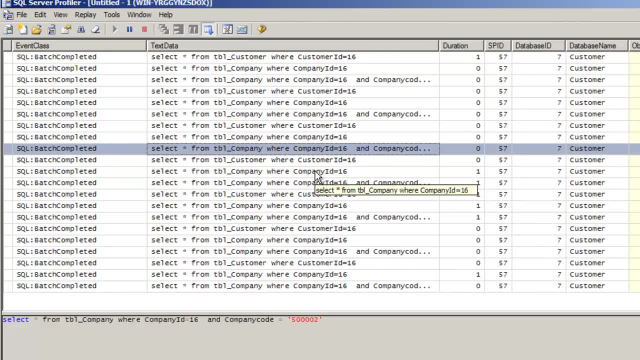 and, if you note over here, he has only captured the select statements which are fired on the customer database because we have put a filter on them. Now, what I would like to know like I would like to save this workload and then I would like to run the tuning advisor on the workload to get suggestions. 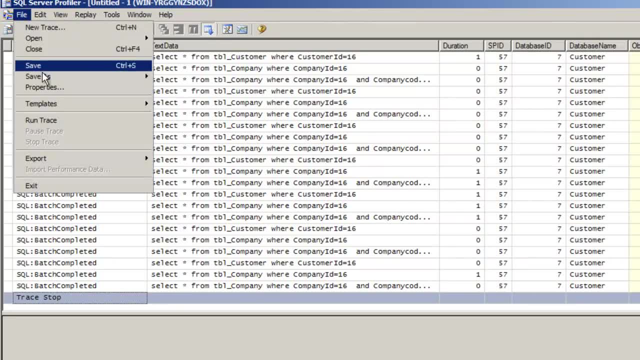 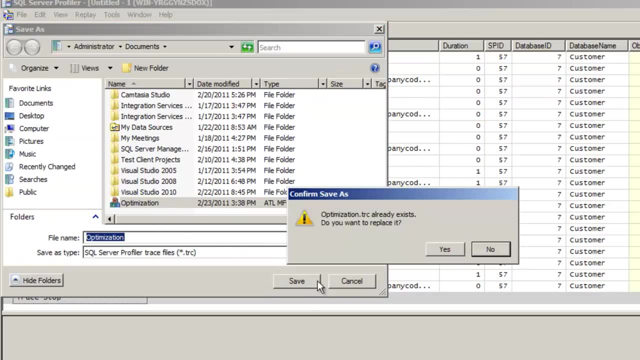 So let me go and stop the profiling for now and let me save this workload file. In order to save this workload file, what you have to do is create it as a trace file. There is a file over here. just go Save As and Trace File. Let me give a nice name to this, called as Optimization. 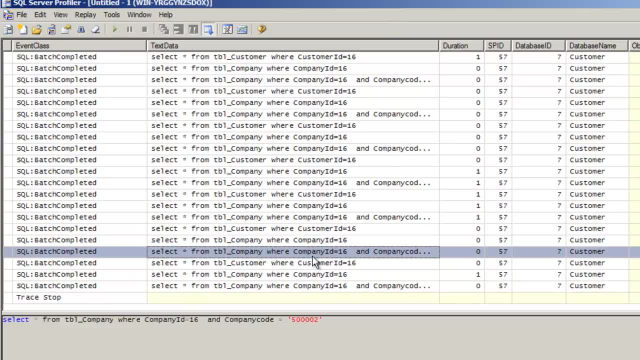 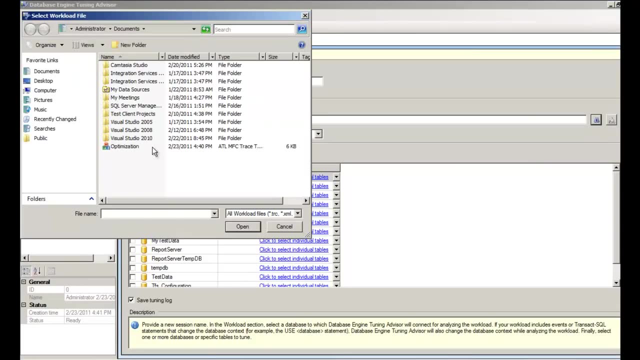 Let me just save this over here. I have saved my workload file. The next step is I have to go and run my tuning advisor on the workload file. Click on Tools, Click on Database Tuning Advisor and provide your work file over here. Browse this and select this optimizationtrc. 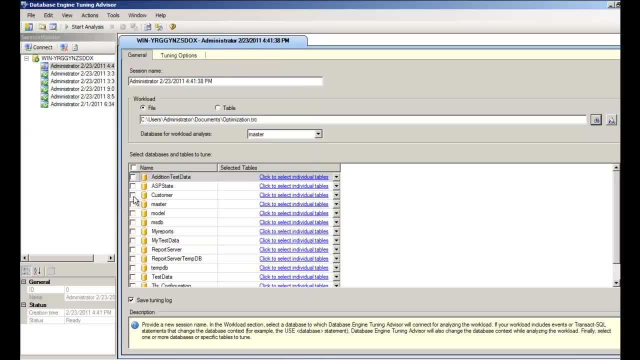 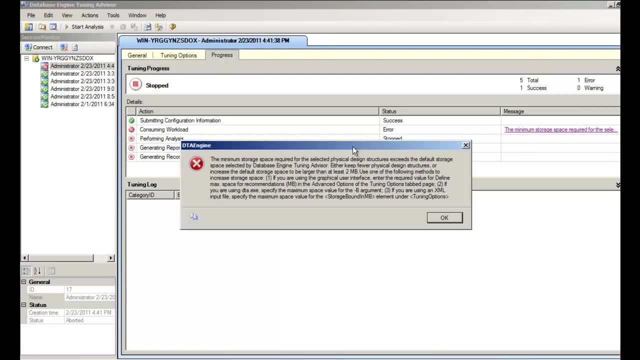 which I had recorded just now. Because I want to run this optimization on my customer database, I will select that database. At the top there is a button called as Start Analysis. just hit on it. There is some kind of error here. It needs some extra space to run your. 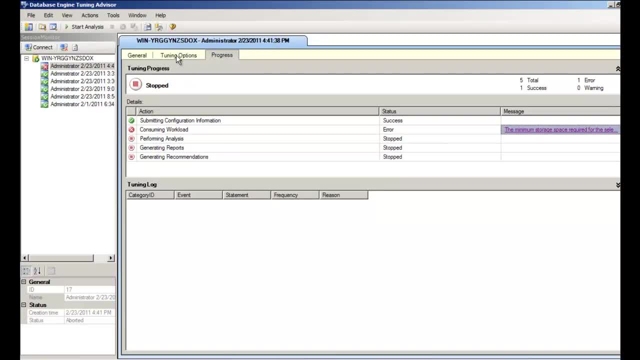 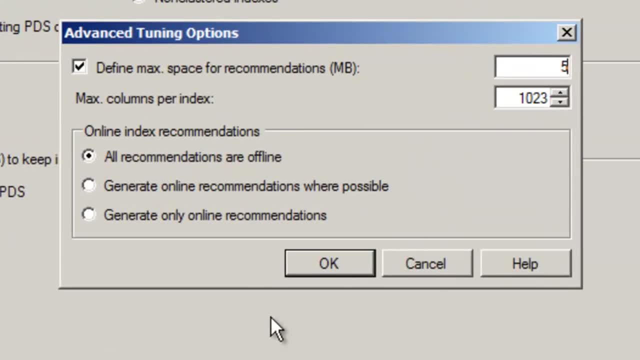 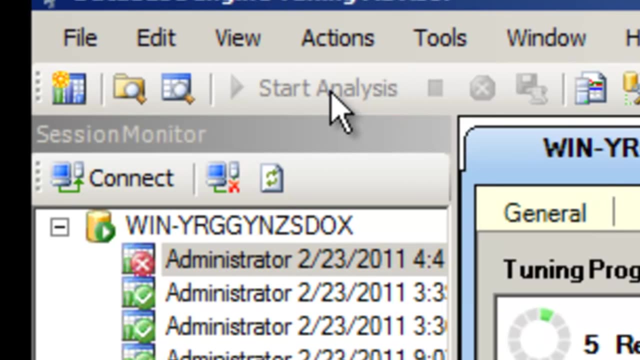 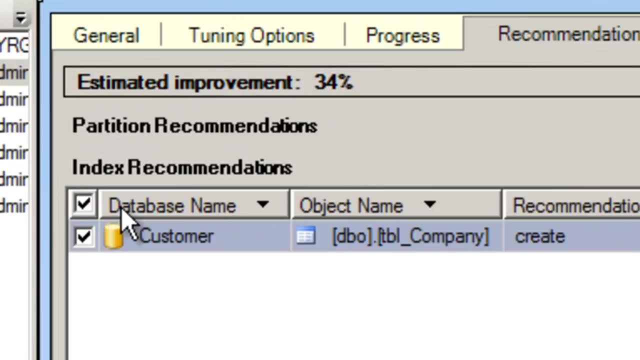 Tuning Advisor, Go to the Tuning Options and go to the Advanced Options. and for the recommendation for the max space. I am just providing 5 MB over here. Let's rerun the analysis. Hit on Start Analysis. again There is an analysis and recommendation. The first thing, what is noticeable here, is that 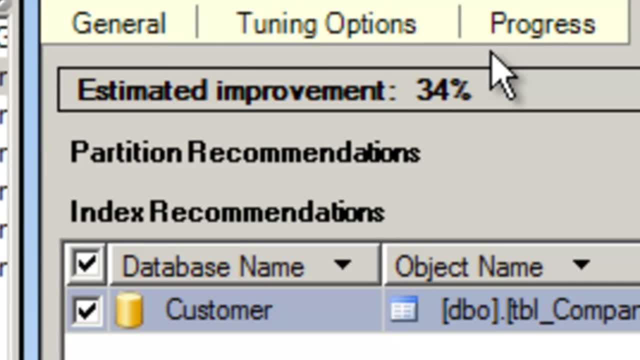 how much percent you can improve if you implement this recommendation. We can see that it has given out one recommendation. We can see that it has given out one recommendation. We can see that it has given out one recommendation. Your performance will improve 34% if you implement this recommendation. 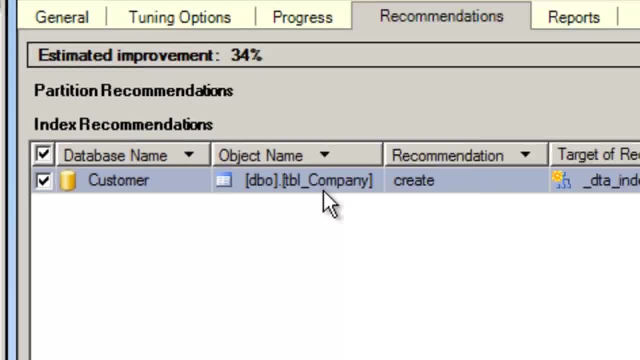 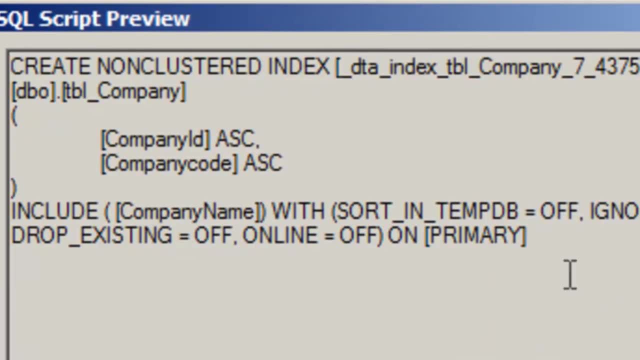 In order to see what the recommendation is. what you can do is currently it has only one recommendation over here. Click on this link here, on the definition link, and you can see the school preview of the recommendation. If you go and create a non-cluster index on the company code and the company id. 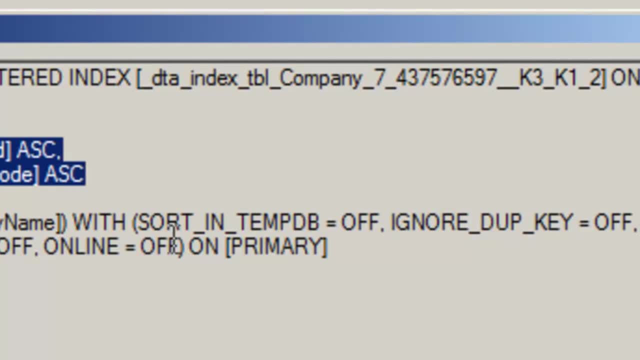 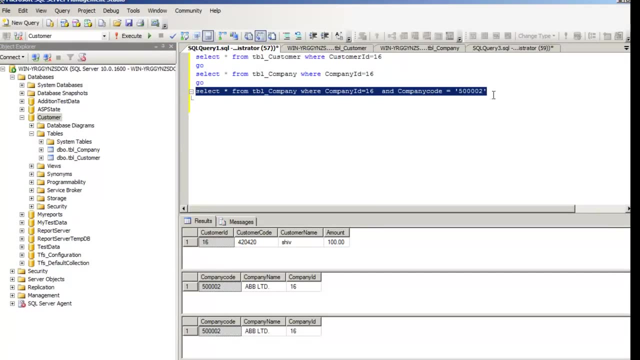 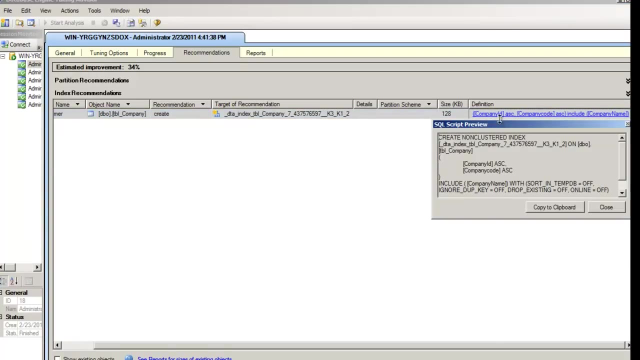 your performance will improve approximately 34%. In our SQL load which we have given, we had one select query which had the combination of company id and company code. By looking at that combination, it has given you a recommendation of creating a combination non-cluster index on both of these columns. 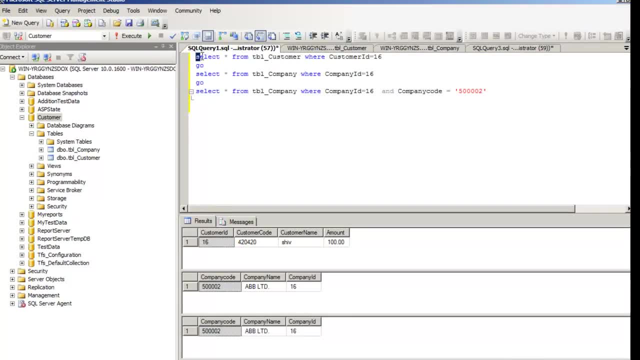 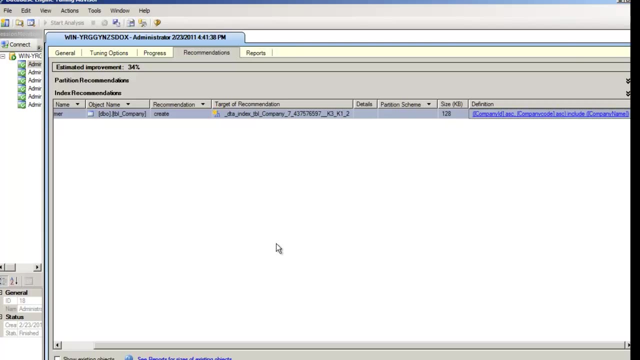 The next question which we will ask is What happened to our select TBL customer? Because it gives recommendations to TBL company, but for TBL customer it has not given any recommendation. One point you need to remember is that the TBL customer had very less number of records. 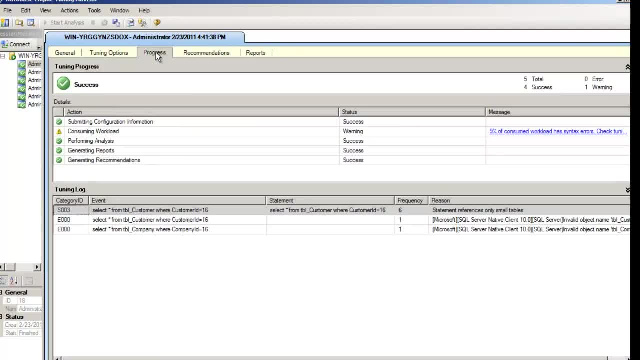 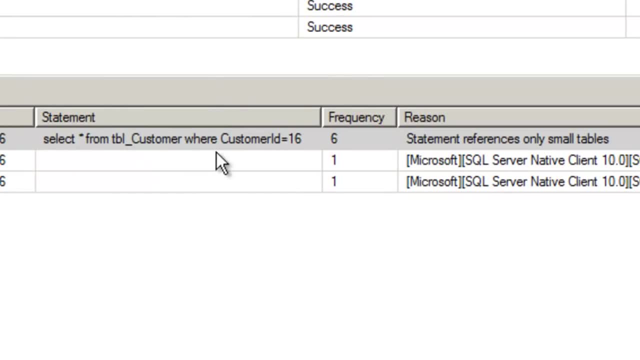 Let me show you what it thinks about the TBL customer. Click on the progress tab here. There is a small statement which is written here. What this statement says is that the TBL customer is very small. The reason is the statement references only small tables. For small tables there is no point in giving index suggestions, because 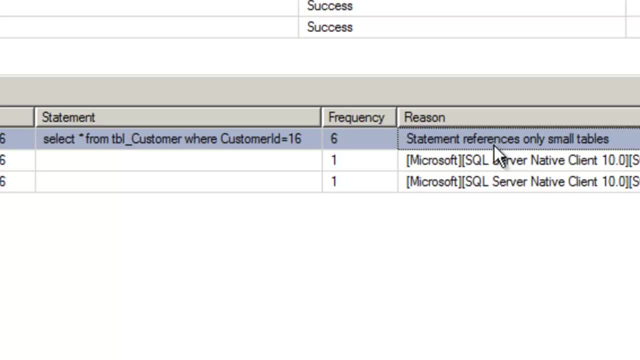 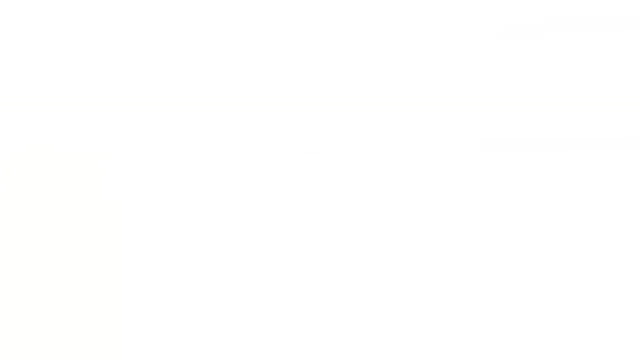 indexes uses B-tree structure or balance tree structure, which is far complex than doing a table scan for small tables Currently. whatever is the scenario is good. probably creating indexes will complicate the matter further. Basically, how it has given recommendations. also how it has given reasons for where he has not given the recommendation. 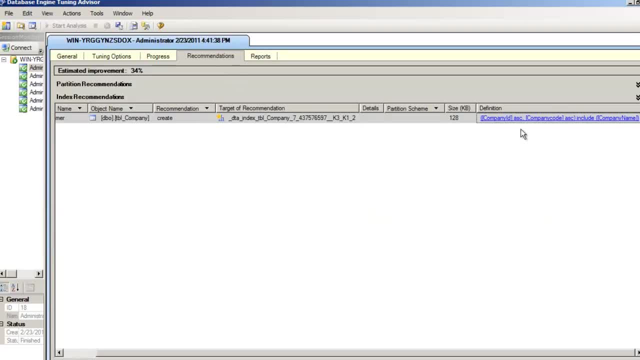 I hope that you have liked this video. In this video, what we did is basically we looked into how to go and create a trace file or a workload file by using the SQL Server Profiler. On the SQL Server Profiler, we basically ran the Index Tuning Wizard. 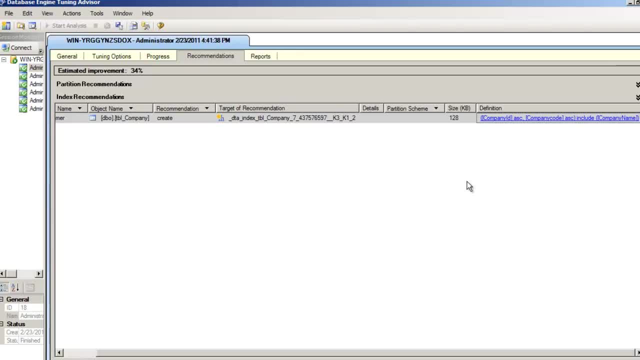 or the Database Tuning Wizard to see how it gives out recommendations and we can then apply those recommendations to improve our performance. I hope that you have enjoyed this part of the video and we will keep continuing the SQL Server Performance tips in this section as we go ahead. Thanks a lot.